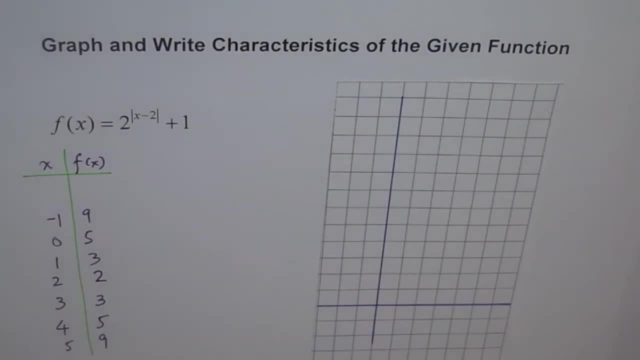 Well, f values are always positive, in this case correct, And it seems at this point 2, 2 is kind of gives us line of symmetry. So what we can do now is plot these values on a graph and then see how it looks like. 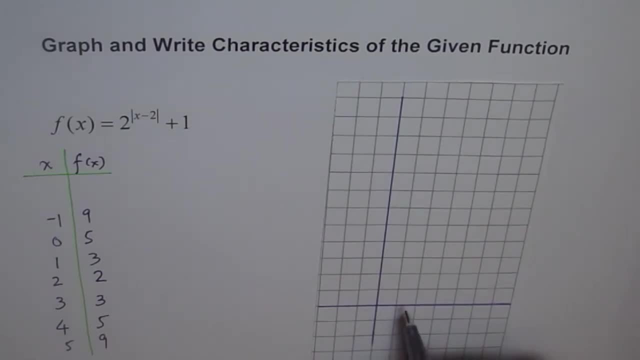 So let's say this is okay. so let's consider this to be 1 positive. This is 1 negative, And let's start from 2,, 2 itself. Okay, so at 2, the value is 2.. So it is 2 here. 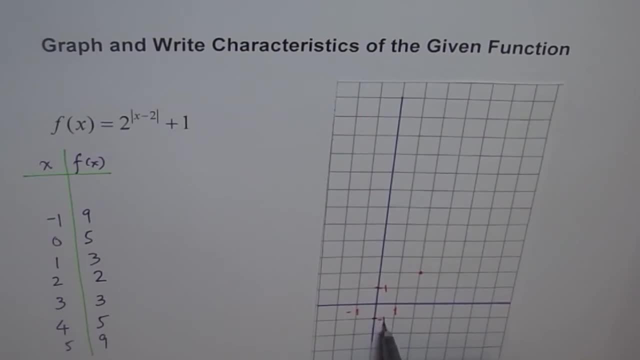 So we have here 1 and here also minus 1, correct, So that's our first point. Then at 3, we have 3.. So at 3, we have 3.. So that's the next value. At 4, we have 5.. 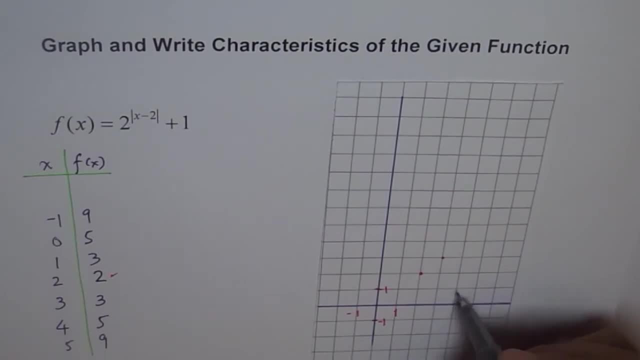 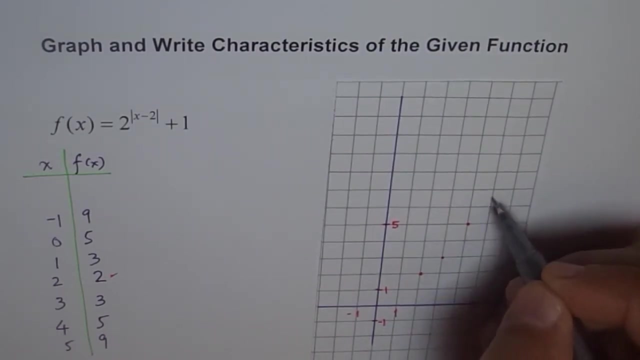 So at 4, the value is 1,, 2,, 3,, 4, 5.. Let's write down 5 here, It helps, And at 5, it is 9. So 1,, 2,, 3,, 4, 5.. Let's say this is 5. 9. So 5,, 6,, 7,, 8,, 9.. 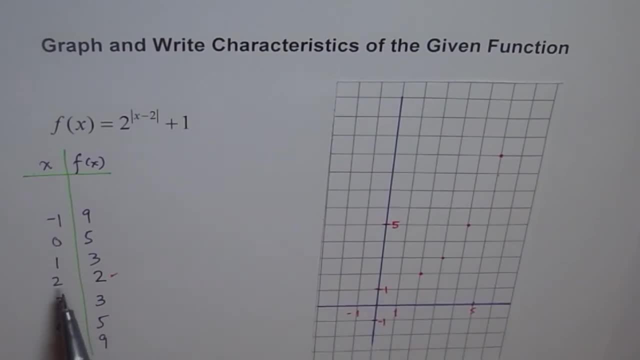 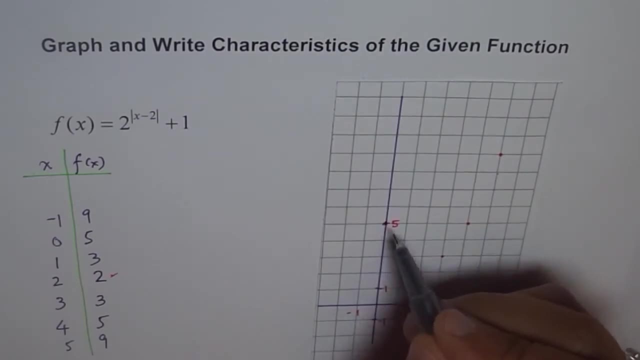 Good, And as we go on this side, that means at 1, it is 3.. So at 1, it is 3.. At 0, it is 5.. We get it here right: At minus 1, it is 9.. It's symmetrical, So like that, correct. 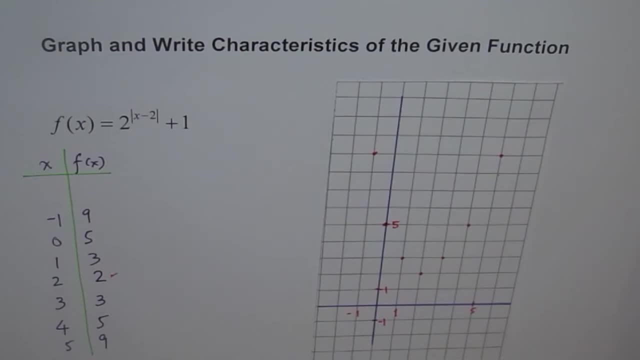 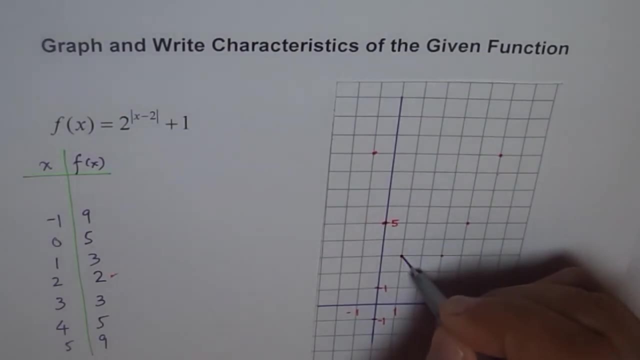 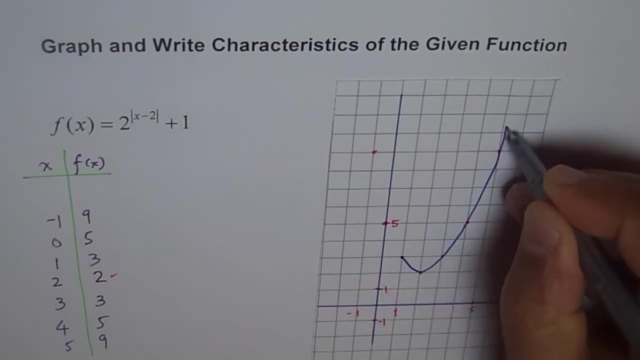 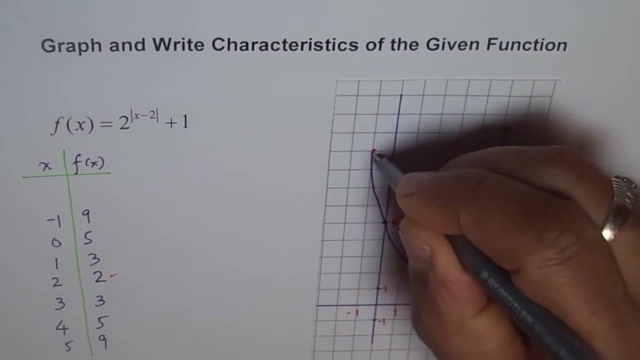 And so on, it will go correct. So, and let's join these points right To get a graph correct. So that is how our function is going to look like. Kind of like this correct Now that's? this is f of x. 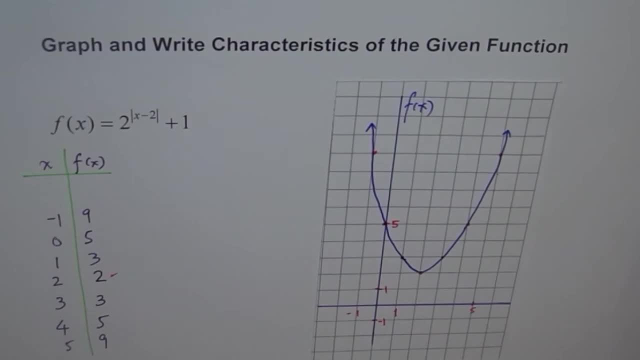 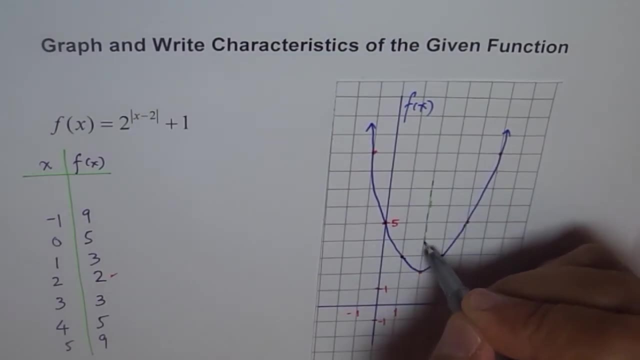 Okay Now, what characteristics do you see here? Well, we see that there is a line of symmetry here, And the line of symmetry is like: at x equals 2.. 2, right. So line of symmetry is at x equals to 2.. 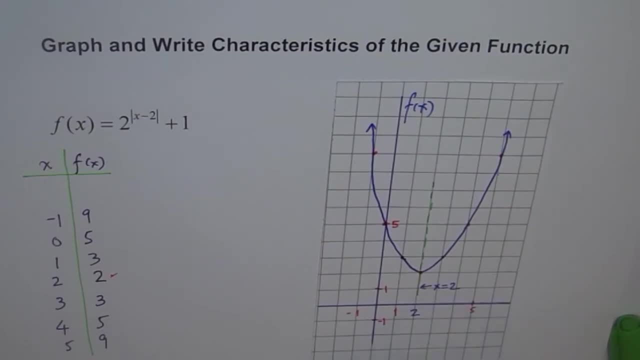 So we have x equals to 2 will give us a line of symmetry. Okay, So the function is decreasing from minus infinity to 2, and just increasing from 2 to infinity. The function is always positive, right, Always positive, And what else? 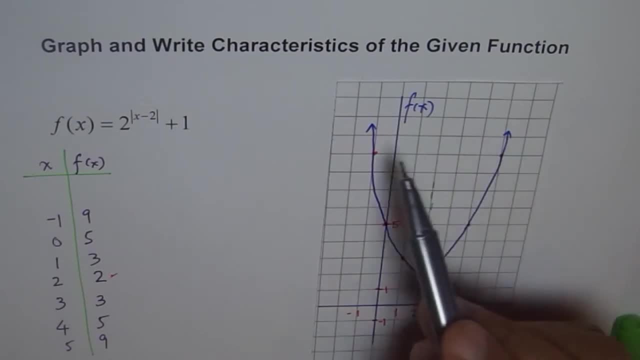 End behavior. So what is the end behavior? As x approaches plus infinity, f of x approaches plus infinity. As x approaches negative infinity, f of x approaches plus infinity, Correct, So that's the end behavior. So these and domain is all real numbers and the range is x greater than or equal to 2.. 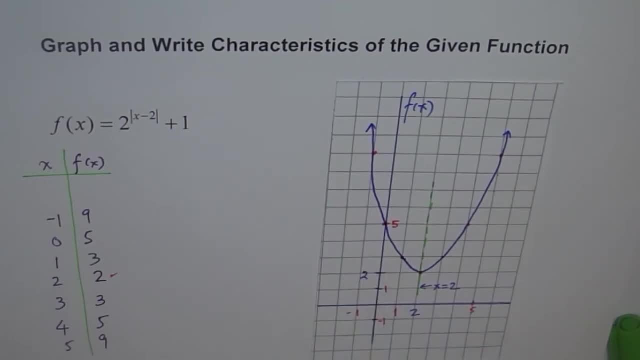 Do you see that? So that value is 2 for us. So these are the characteristics of the given function. So what we can write here, some of our characteristics, and these are. let me just put a line here and then we'll write down the characteristics here as: 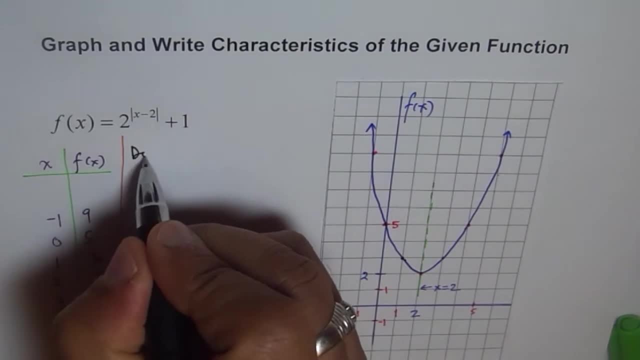 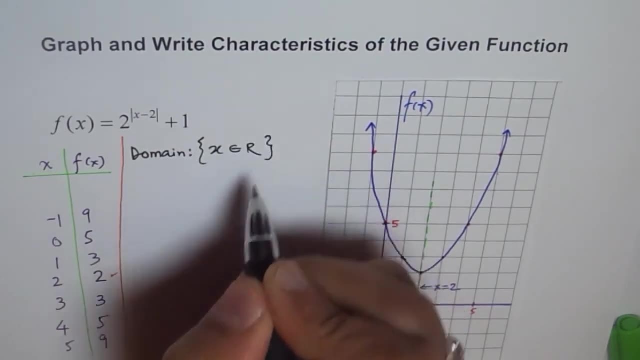 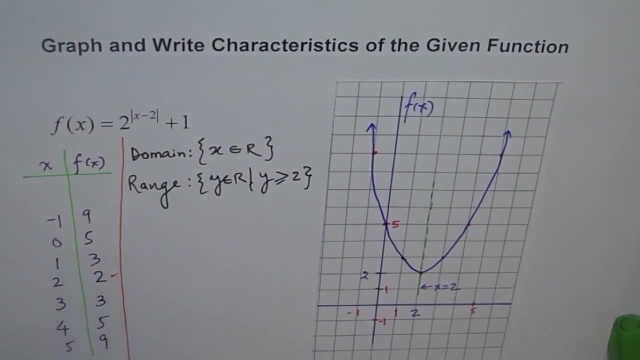 first-trick domain is: x belongs to real numbers. right, There are no restrictions. correct Range: y belongs to real numbers, but y is greater than or equal to 2.. Is it okay Now end behavior. End behavior is: x approaches negative infinity. 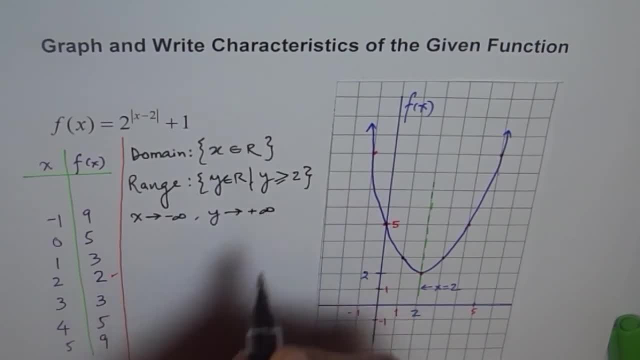 y approaches positive infinity And as x approaches positive infinity, y approaches positive infinity, Correct. And it is increasing interval and decreasing interval. we'll say Increase from increases from 2 to infinity, right, And decreases from increases from minus infinity to 2, correct. 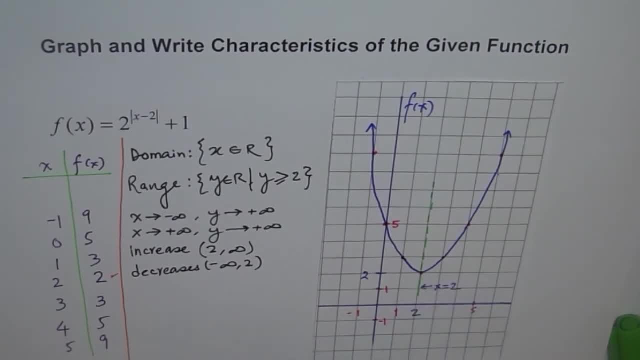 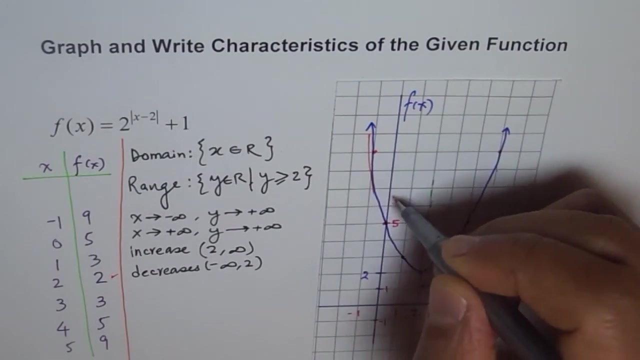 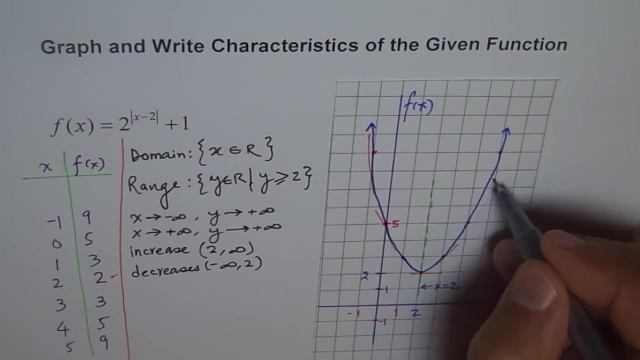 It has now. if you see rate of change all along, because the shape is like this, you see rate of change. Let's discuss rate of change of this function. That's kind of important right Here is negative, very negative, less negative, 0, positive, more positive. do you see?